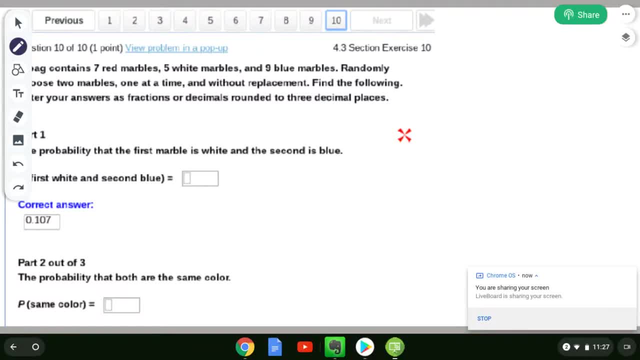 I'm going to go ahead and work part two of this problem. So we've got a bag that has seven red marbles, five white and nine blue. So altogether that gives me my n, which would be. so n is 12. 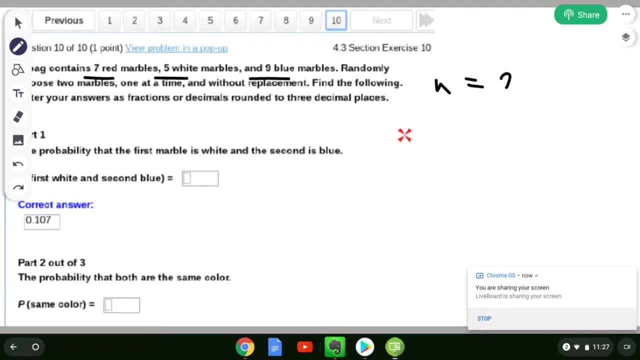 plus 9 is going to be 21.. So, as we're working this part two, it says we want the probability that are both the same color, So to get them both the same color. that means that we're really looking at the probability that these two marbles we're drawing- two of them are going to 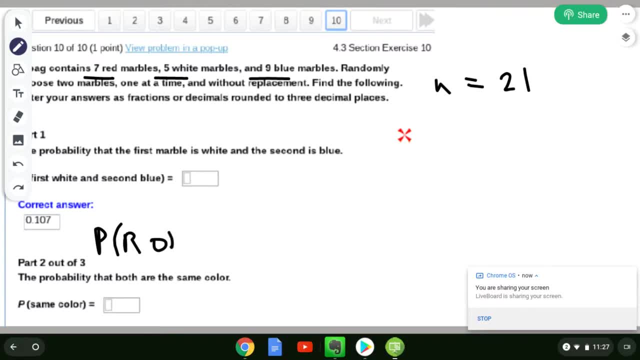 be red, or so we're using that word, or in between, or both are white or both are blue. So we really have this or probability, and in probability we've got these separate cases. so we're going to connect those probabilities with a plus sign. So as we go through and work through the math, we've got 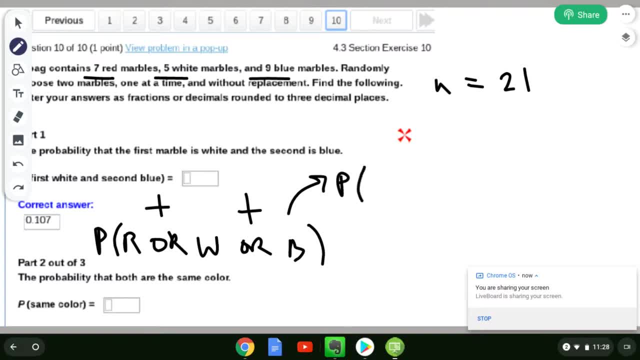 three different probabilities to compute. So the probability that they are both red, so a red and a red. I'm going to write my little and sign there. so a red and a red, or which is going to be, plus the probability that they're both white, which is going to be white and white. 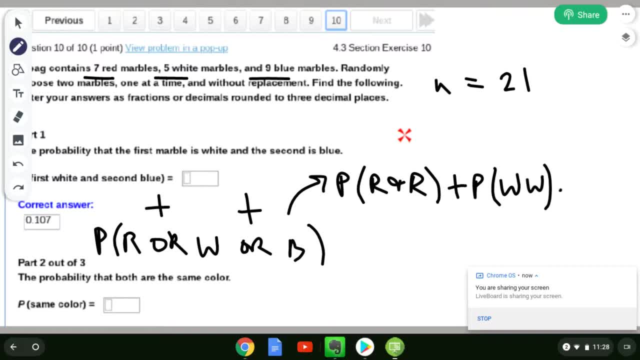 I'm just going to write ww here plus for, or the probability that they're both blue, So I've got just enough room to write a b and a b there. So we're going to use our, and, which means that we'll. 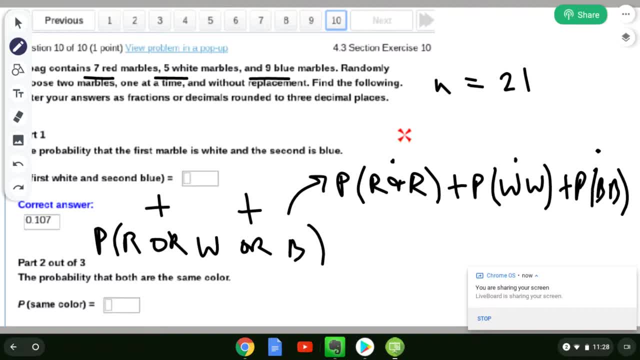 have two red and a b, but then adding each of those separate probabilities together. So let's start with the probability that we've got one that's red. So first of all, let's see we're drawing both of these randomly. We're drawing two marbles, one at a time, without replacement. So that's important. 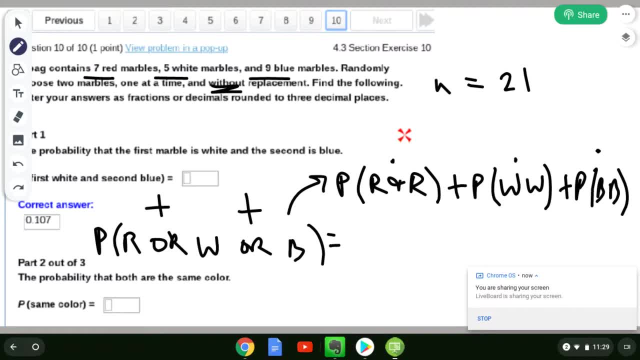 That means once we draw one marble we've got 20 left in the bag. So we're going to go through case number one. These are separate cases, So the probability that the first one is red, red we've got to match those. So the probability that the first one is red is going to be seven out of 21.. 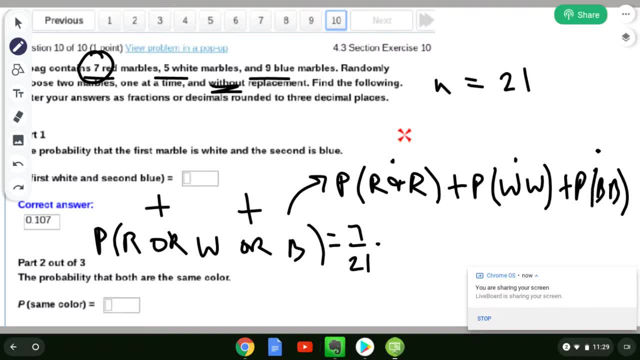 And we want the second one to be red as well. Well, we already drew one red, so that means we've got six red left and we've got 20 left in the bag. Now we go on to the second probability. So completely.